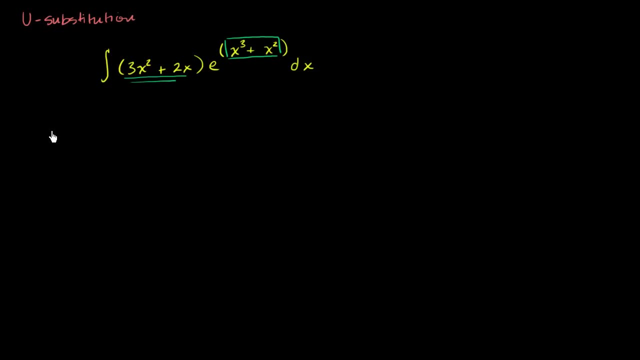 where I also see its derivative being multiplied. I can set that equal to u. So I can say u is equal to x, to the third plus x squared. Now, what is going to be the derivative of u with respect to x? du, dx. 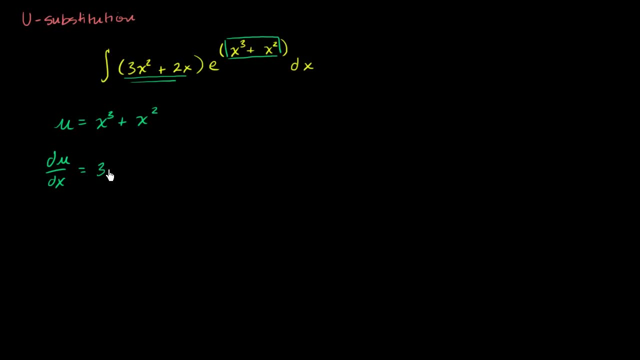 Well, we've done this multiple times- It's going to be 3x squared plus x squared, That's 2x. And now we can write this in differential form: And du dx. this isn't really a fraction of a differential of du divided by a differential of dx. 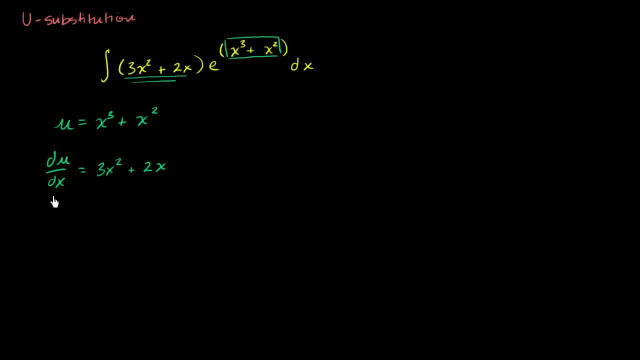 It really is a form of notation, But it is often useful to kind of pretend that it's a fraction And you could kind of view this if you wanted to just get a du, if you just wanted to get a differential form over here. 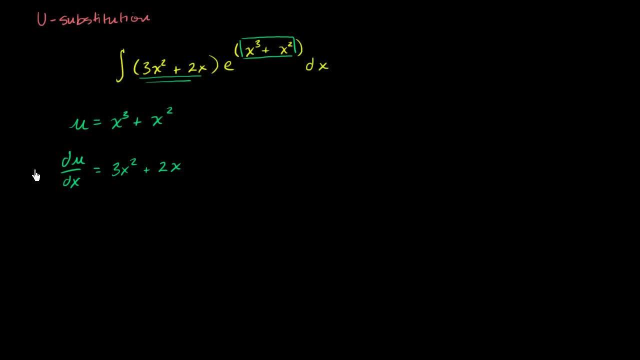 How much does u change for a given change in x? You could multiply. You could multiply both sides. You could multiply both sides times a dx, So both sides times a dx. And so if we were to pretend that they were fractions and it will give you the correct differential form, 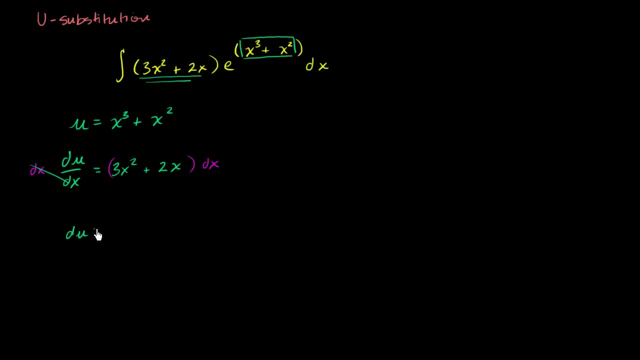 you're going to be left with du is equal to 3x squared plus 2x dx. Now, why is this over here? Why did I go through the trouble of doing that? Well, Well, we see, we have a 3x squared plus 2x. 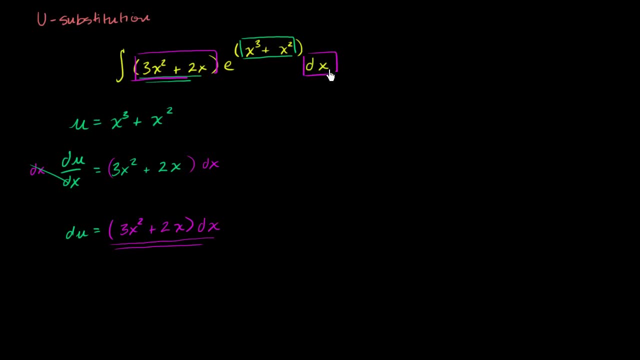 And then it's being multiplied by a dx right over here. I could rewrite this original integral. I could rewrite this as the integral of: let me do it in that color of 3x squared plus 2x times dx times e. 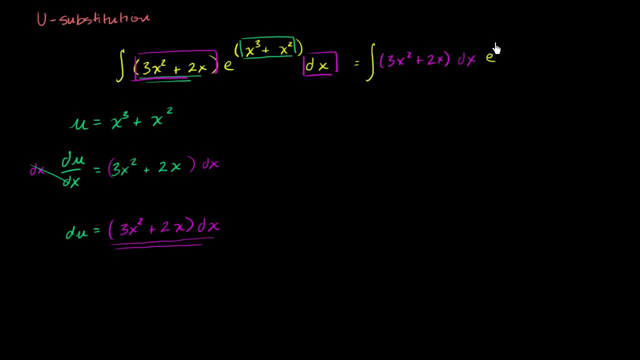 Let me do that in that other color. Times: e to the x to the third, plus 2x Times e to the third, plus 2x squared, plus 2x squared, plus 2x squared. Now what's interesting about this? 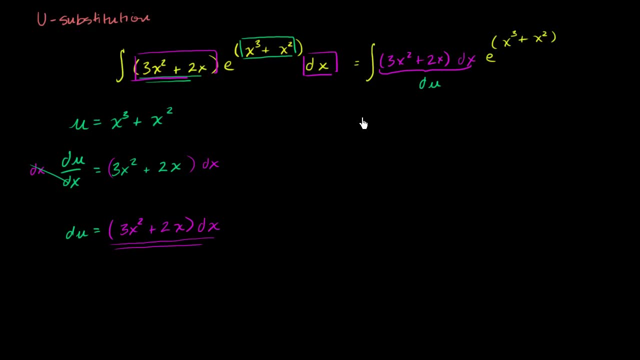 Well, the stuff that I have in magenta here is exactly equal to du. This is exactly equal to du. And then the stuff I have up here: x to the third plus x squared. that is what I set u equal to. That is going to be equal to u.